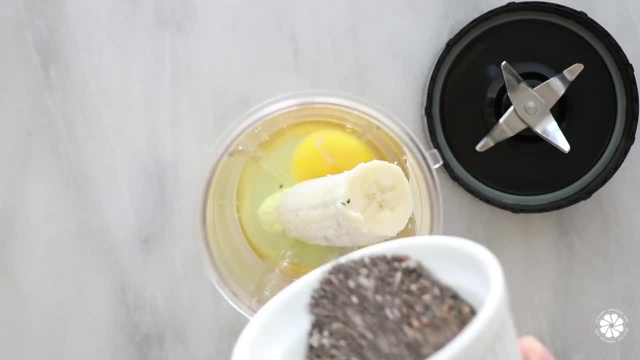 chia seeds and flax seeds and blueberries. Add all of your ingredients into a blender, except the blueberries, and then blend. Pour batter vaporously into a small bowl and then lower the oven temperature to 160 or Tae level, Whenever you have all ingredients in the aprender at room temperature. 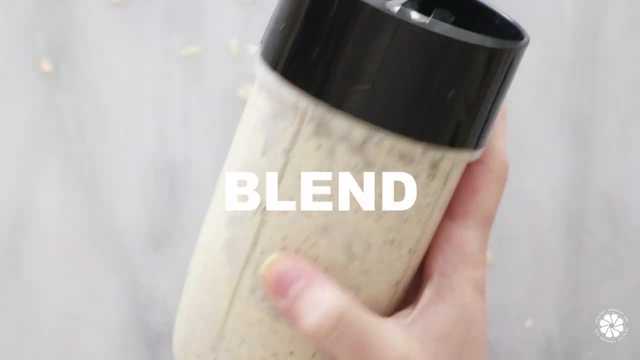 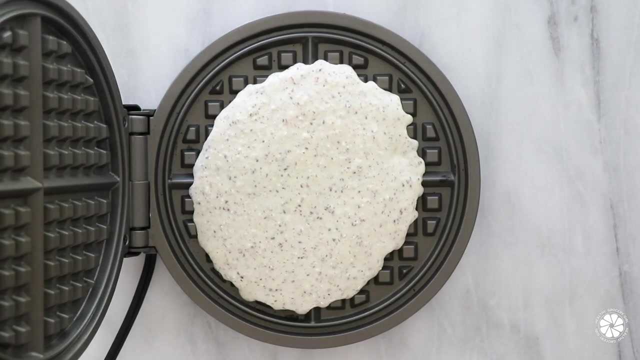 immerse in water slowly so that you can have enough but no plchar soy paste. Mix thoroughly to Agent fait sor Deus. And let rest for 30 minutes. Then add piece by piece into the bowl. �� into a waffle maker and top with blueberries. Serve as you like. For Ella, we cut into sticks 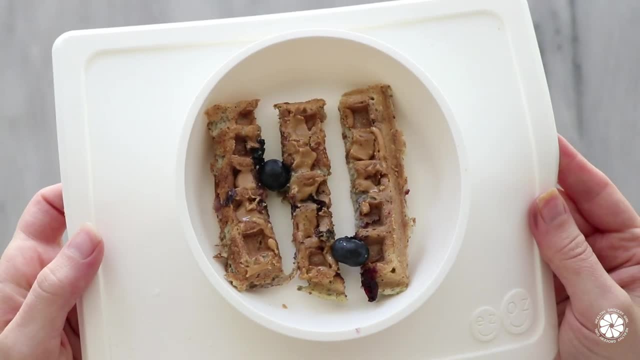 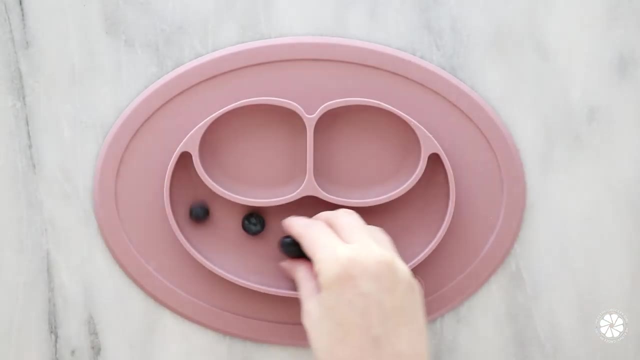 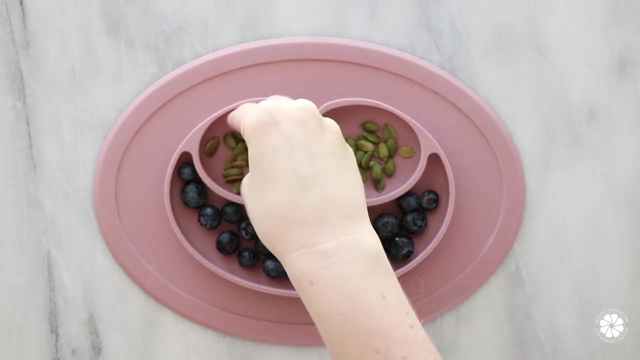 and top with almond butter. This is one of Ella's favorite snacks- Blueberries, which are rich in antioxidants, and pumpkin seeds, which have protein, fiber, healthy fats and zinc, which supports immune health. I buy organic, raw pumpkin seeds. When Ella was younger, I would squash the 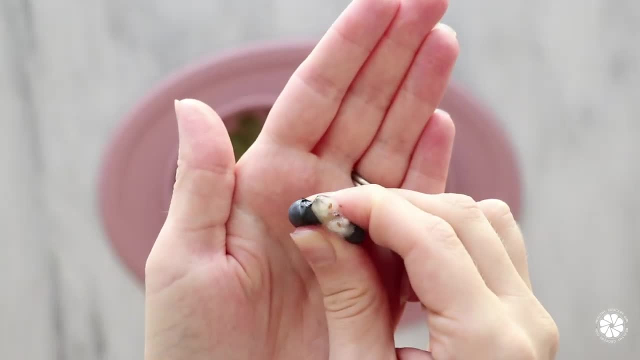 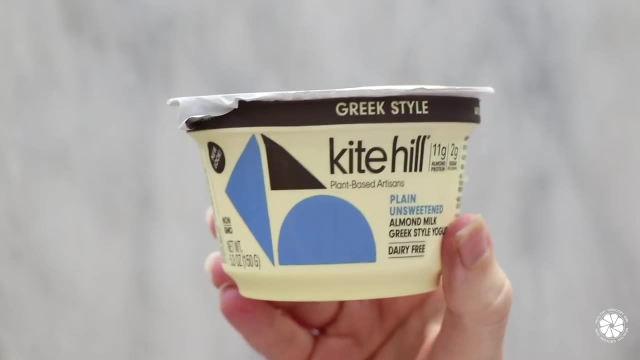 blueberries so they would be easier for her to eat, but now that she is older and has more teeth, she's able to consume the blueberries just as they are. Another favorite is yogurt. We love this dairy-free almond milk yogurt from Kite Hill. It has 11 grams of protein, no added sugar and 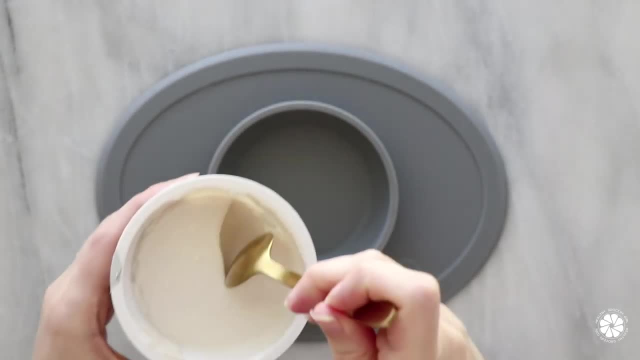 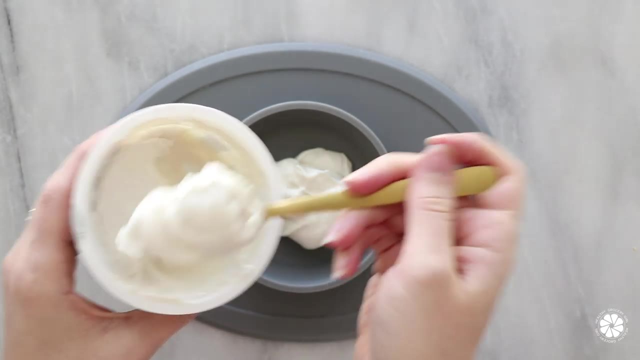 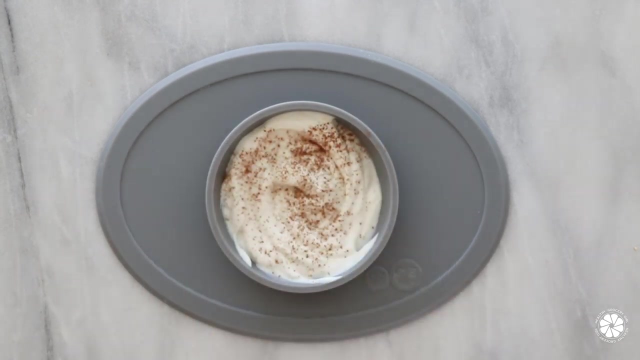 probiotics. We buy the unsweetened and the unsweetened vanilla, which is also really delicious. Greek yogurt is easier for toddlers to eat than traditional yogurt because it's thicker and it sticks on a spoon. I mix in some cinnamon and she also loves yogurt with a side of blueberries. 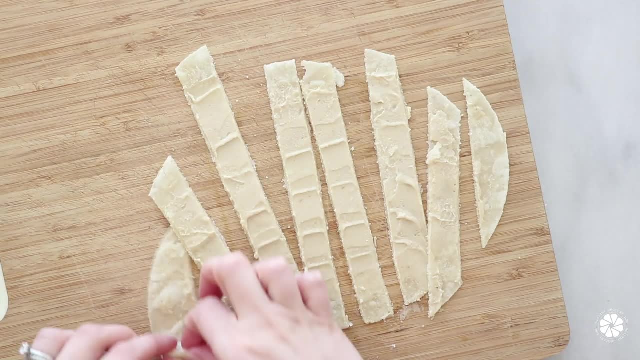 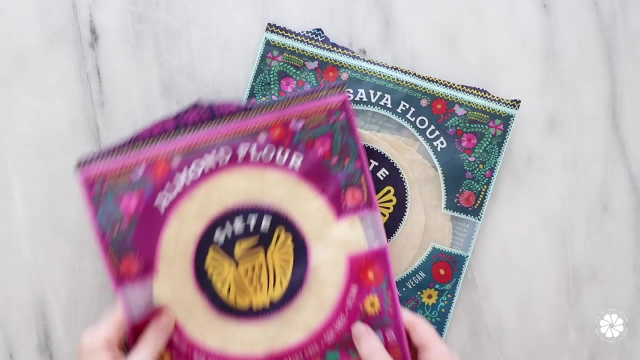 Hummus roll-ups are a big win in our house. I take a tortilla, add some hummus, cut into strips and roll into smaller bite-sized pieces. These are the tortillas that we often eat as a family. They're made with either almond. 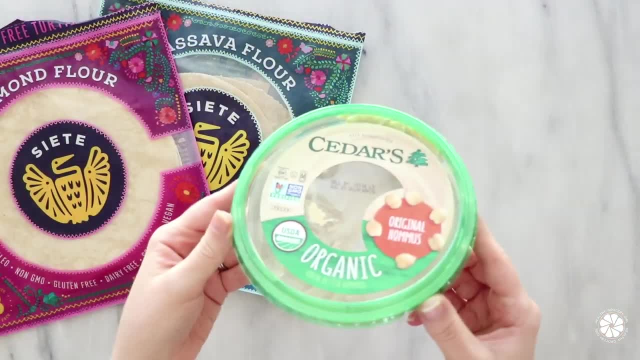 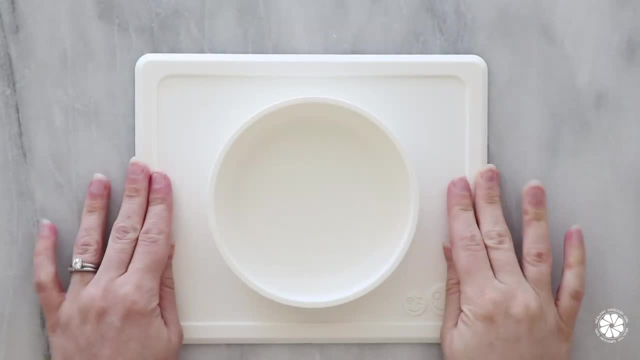 or cassava flour, so they are gluten-free. but any tortilla will work And this is our current go-to. hummus. Pesto pasta is one of our family favorites. The pasta is made from legumes, so it's high in protein. 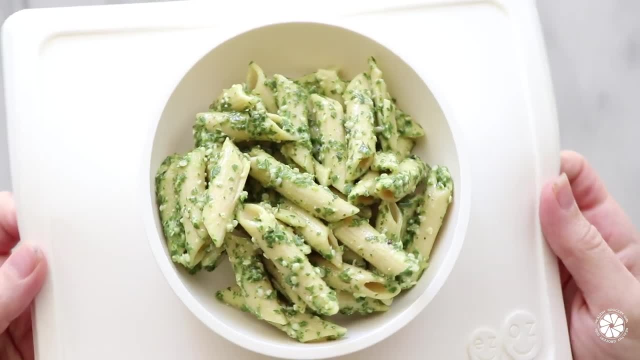 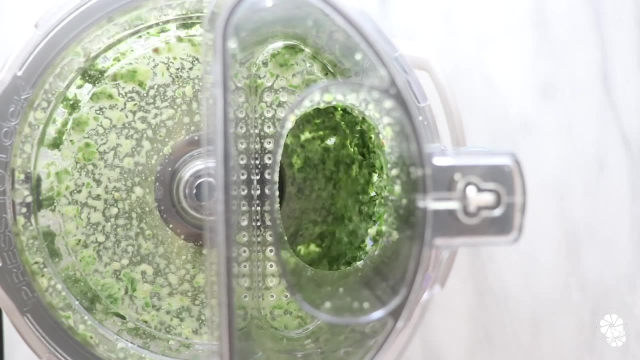 and gluten-free. The pesto is dairy-free and full of healthy fats and nutrients. I shared the full recipe for this pesto pasta on our YouTube channel already, so I will put a link below for that recipe video. below in the video description. 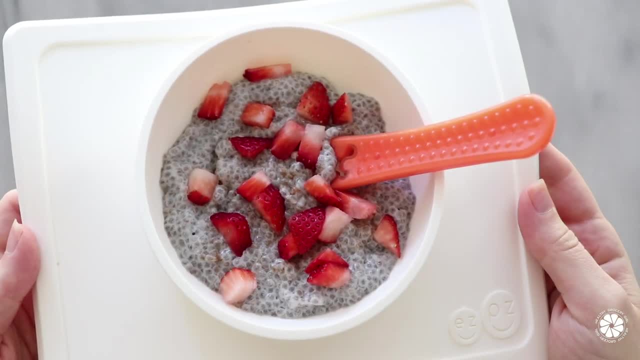 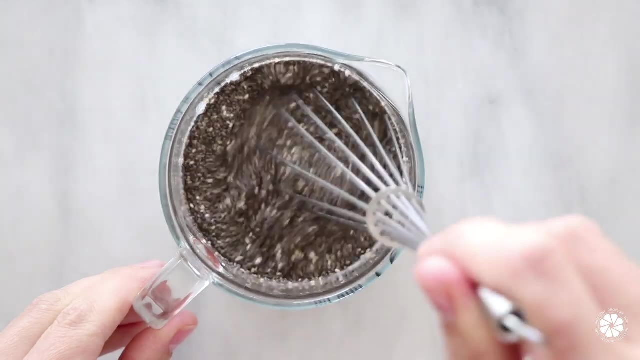 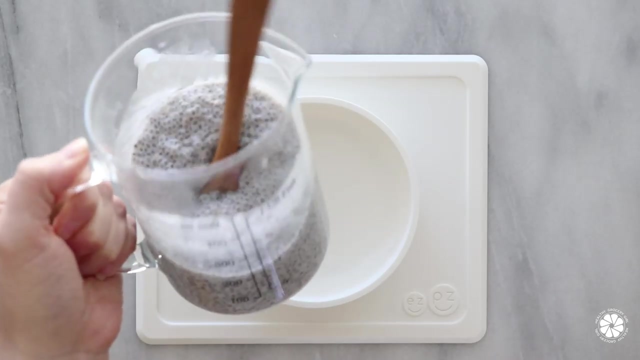 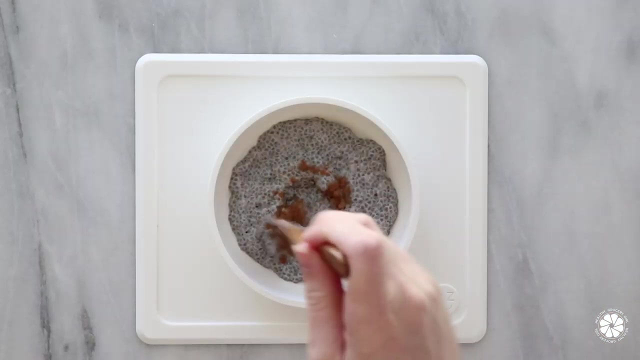 My daughter loves chia pudding. This is made with 1 cup of non-dairy milk and 1 quarter cup of chia seeds, Stir together and then let set in the fridge for 4 hours. I top with cinnamon and she sometimes likes fruit mixed in or on the side. 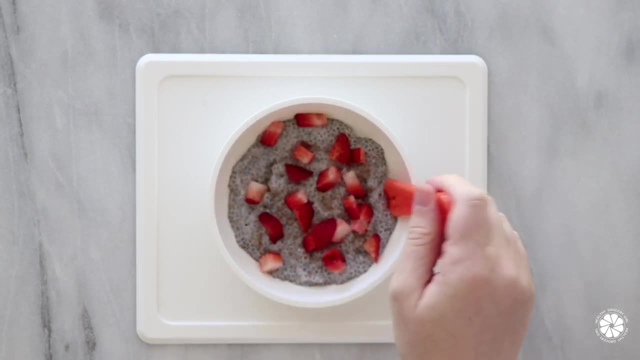 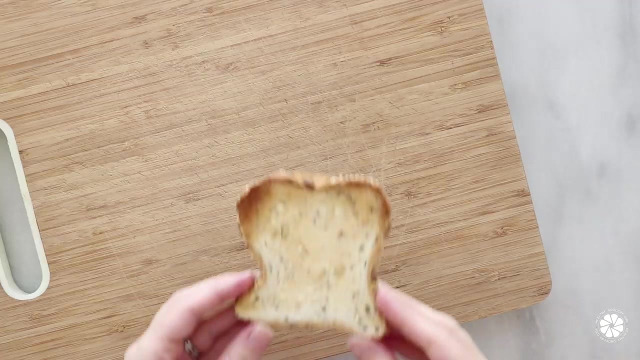 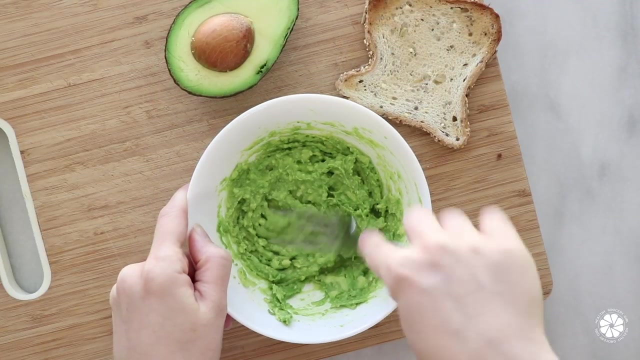 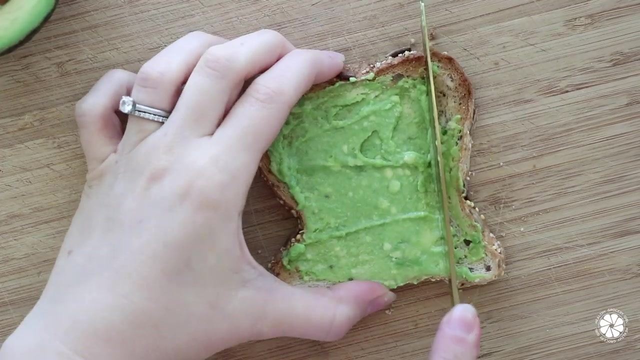 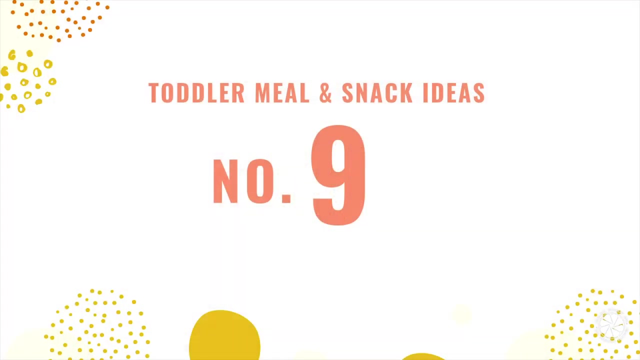 Another snack we love is avocado toast. I start with a piece of bread lightly toasted, then mash a ripe avocado, Spread avocado on top of toast and I cut into little sticks that my daughter can easily grab and enjoy. These spinach muffins are a favorite in our house. 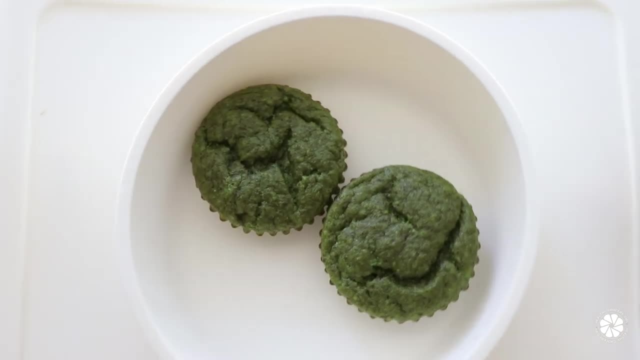 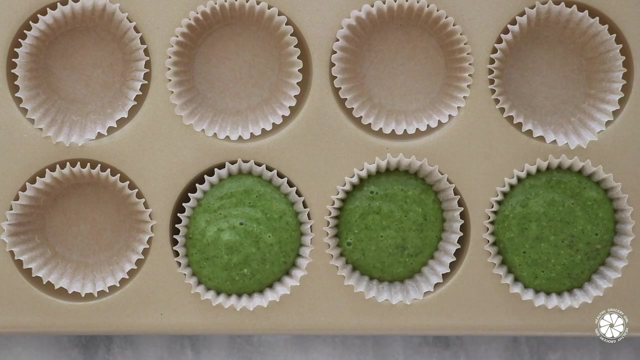 They're made with just a few simple ingredients that you add to a blender, blend and then bake. I've also shared this full recipe on our YouTube channel already, which I will link below in the video description box. I make a big batch of these muffins every single week. 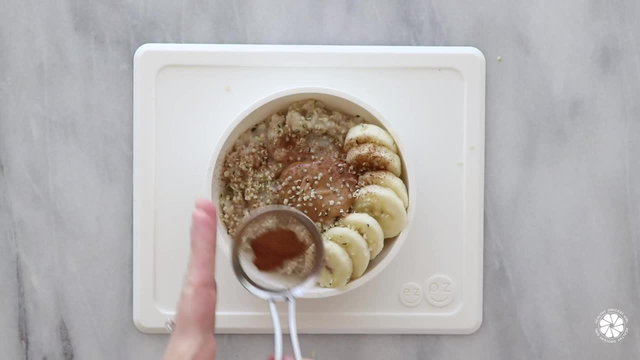 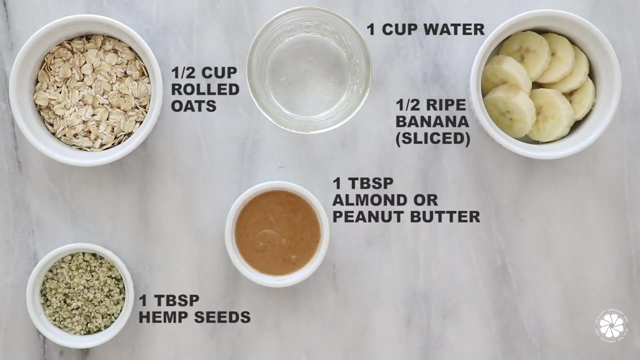 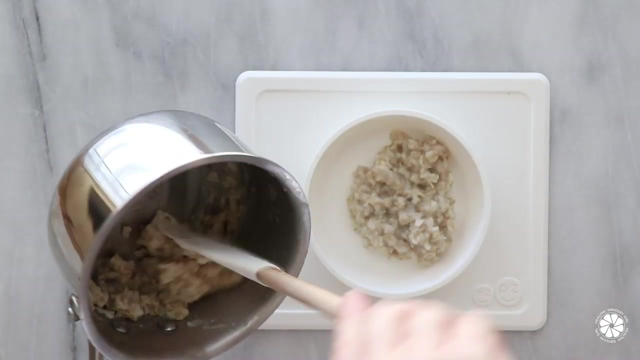 Oatmeal is a breakfast staple in our house. Our go-to recipe is organic rolled oats, water, banana, hemp seeds, almond or peanut butter and cinnamon. Start by adding the oats and the water into a pot and cook on the stove top. 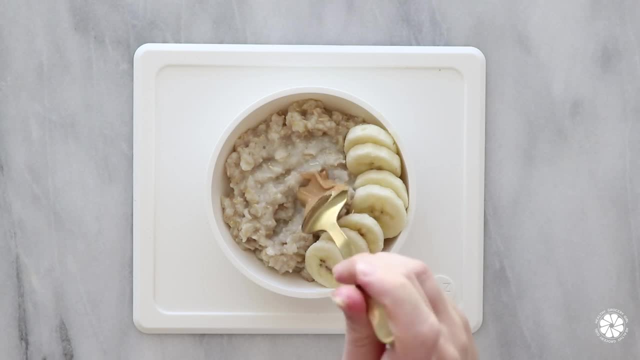 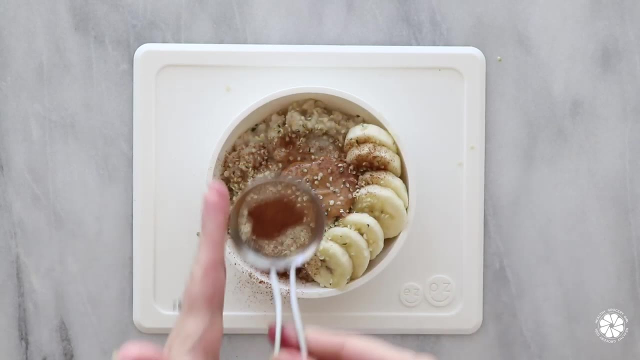 Then add your toppings and enjoy. I got a little carried away with the amount of almond butter I added onto this oatmeal when filming. We would not give Ella such a large serving of almond butter, But we do add a little dollop and we mix it in. 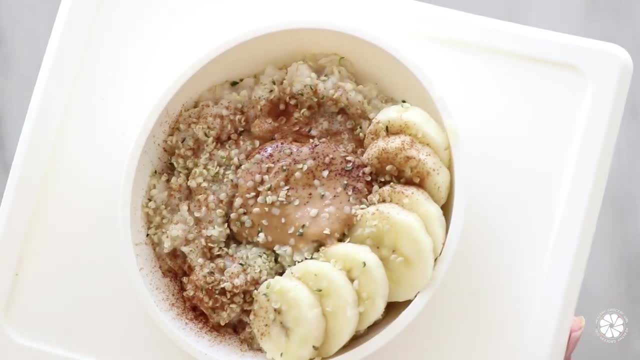 For more details on the recipes, meals and snacks I shared with you today, and also on our favorite eating in kitchen gear, make sure to check out the links below in the video description box. Thank you so much for watching today and for subscribing to our channel. 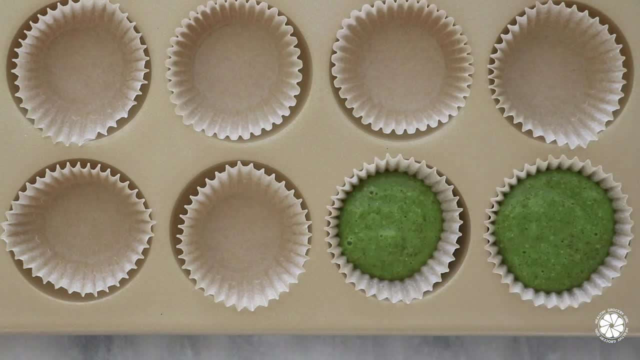 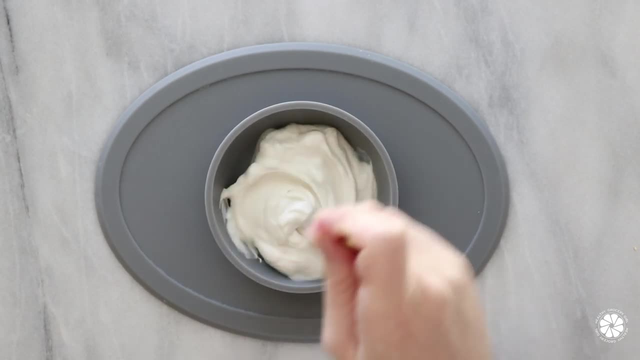 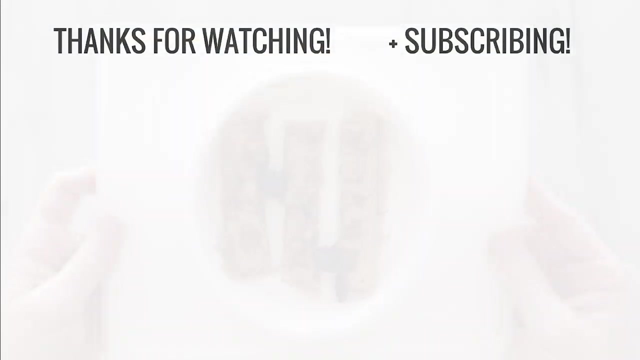 I hope you guys are having a great day and I will see you in the next video. Bye, Bye.